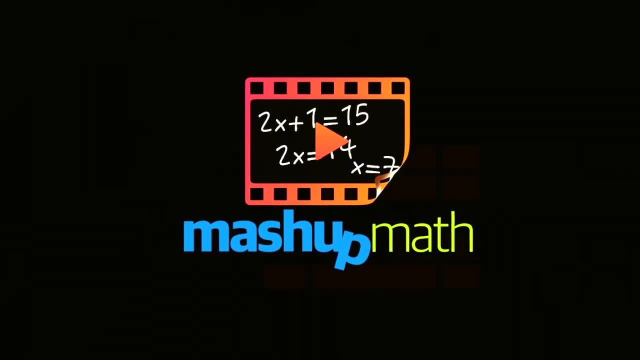 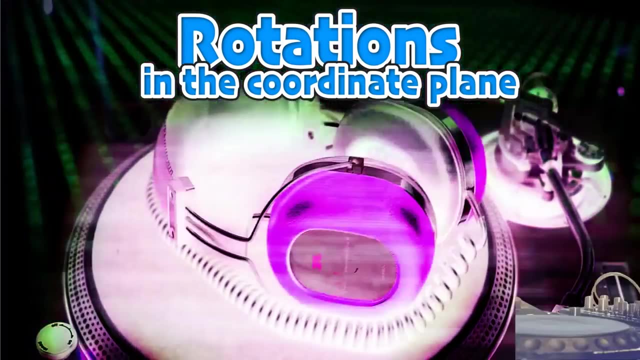 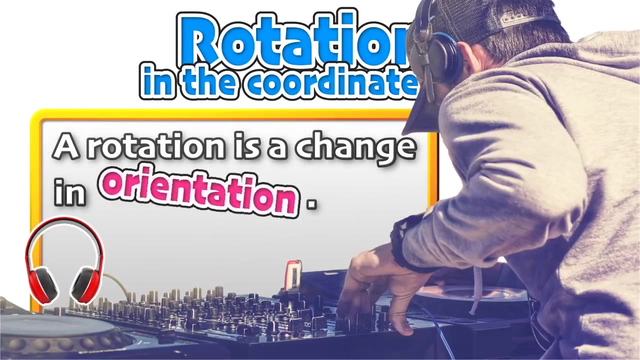 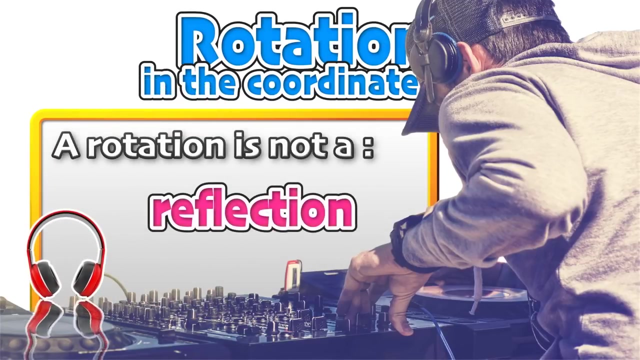 So let's kick off this lesson on rotations in the coordinate plane by watching these headphones spin around on a record. In geometry, we call a rotation a change in orientation. Note that a rotation is not a change in size and that rotation should not be confused with reflections. 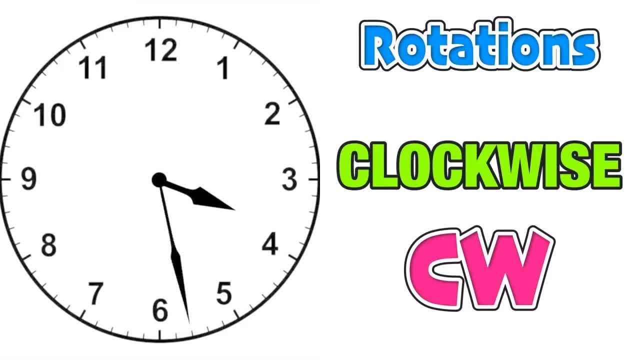 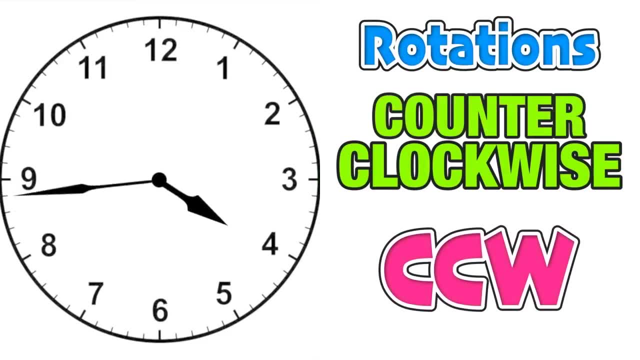 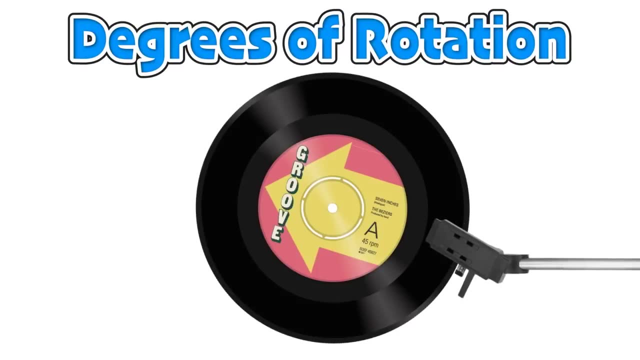 Now we are going to reference two directions for rotations. Clockwise rotations move the same way that the clock does, and counterclockwise rotations just move in the opposite direction that the hand of a clock would normally move. Now, in addition to the direction of a rotation, 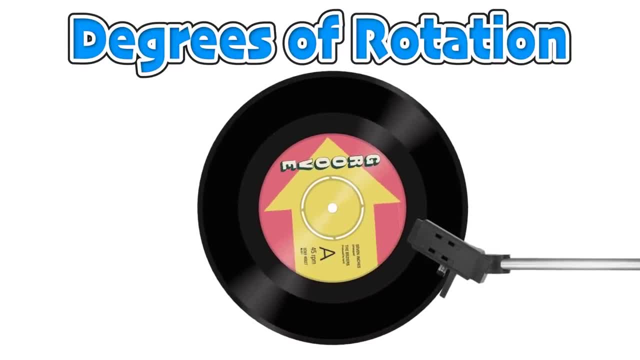 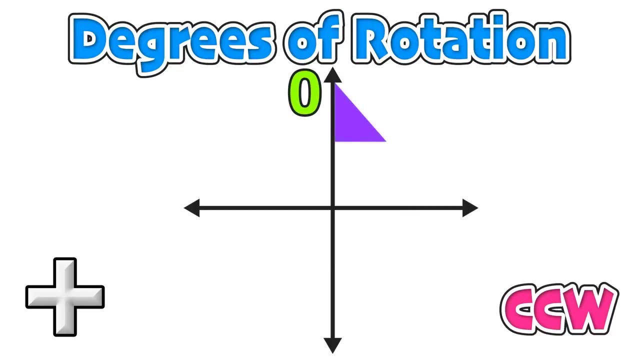 either clockwise or counterclockwise. we are also going to reference rotations in terms of degrees, Just like this circular record. we are moving in a circular rotation, so our degrees are going to be between 0 and 360.. Now, a positive degree of rotation is a counterclockwise movement. So we start with a figure and making 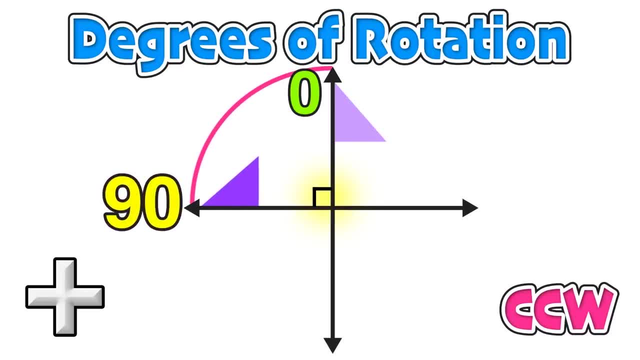 one quarter turn is equivalent to a 90 degree rotation. A second quarter turn is adding another 90 to that. 90 plus 90 equals 180. So this would be 180 degree rotation. A third quarter turn would be adding another 90. This would be a 270 degree rotation. 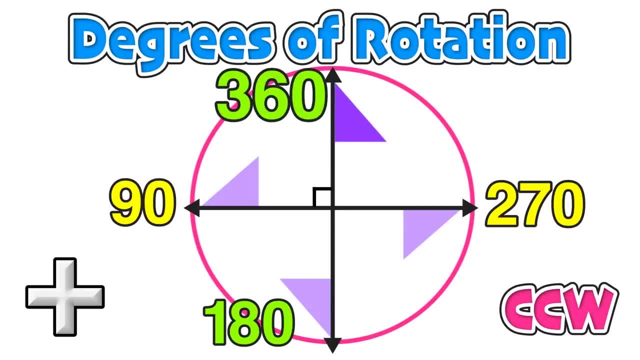 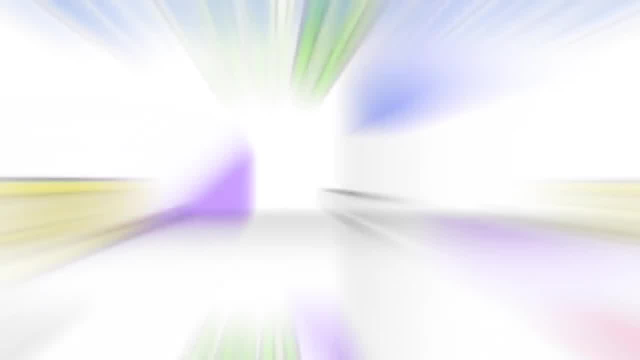 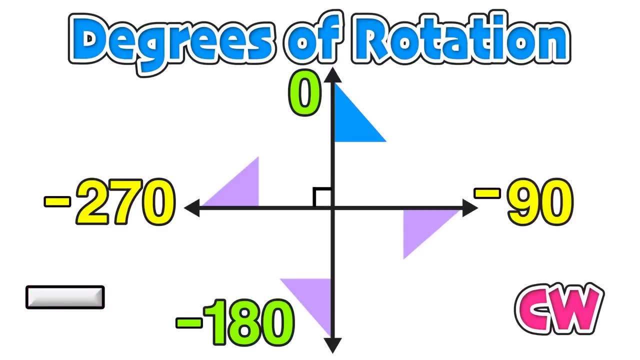 A final quarter turn brings the figure back to where it started and completes the full 360 degrees. Now, if we rotate in the opposite direction, then the figure will be at the same time as this time clockwise. we will see that our rotations will be negative values. 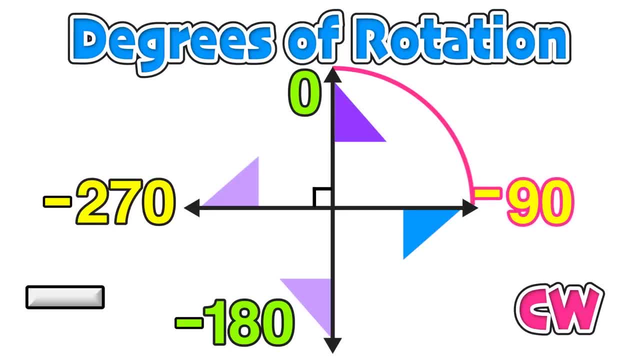 So a negative 90 degree rotation is one quarter turn in a clockwise direction. A second quarter turn clockwise would be negative 180, which, we notice, puts it in the same location as positive 180, so a 180 degree rotation does not matter whether you move clockwise. 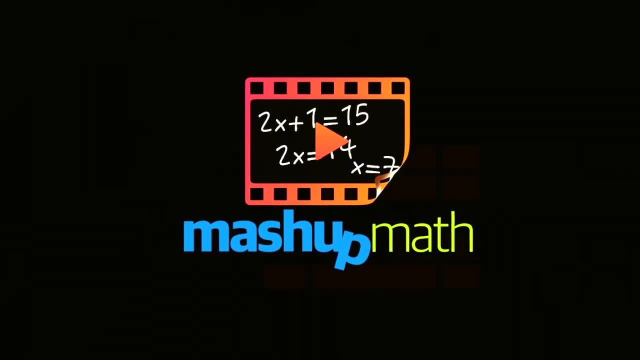 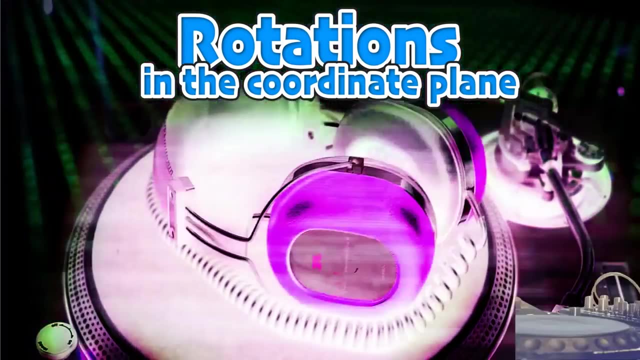 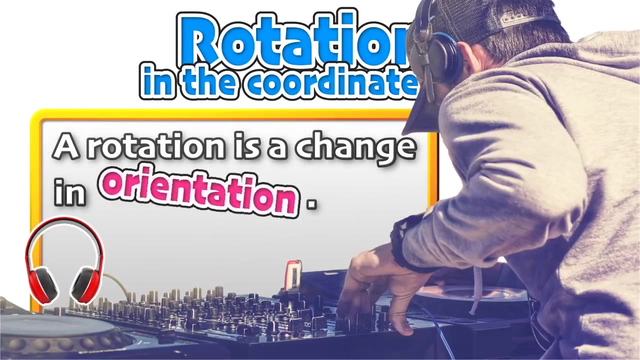 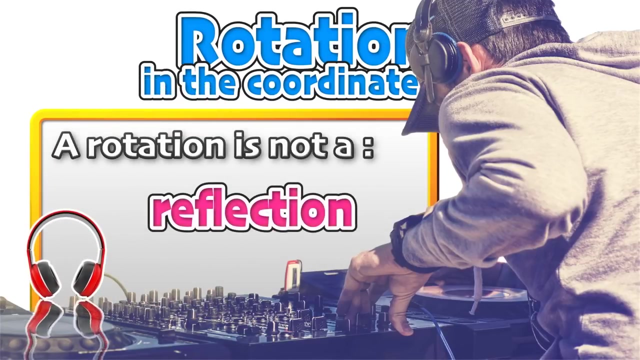 So let's kick off this lesson on rotations in the coordinate plane by watching these headphones spin around on a record. In geometry, we call a rotation a change in orientation. Note that a rotation is not a change in size and that rotation should not be confused with reflections. 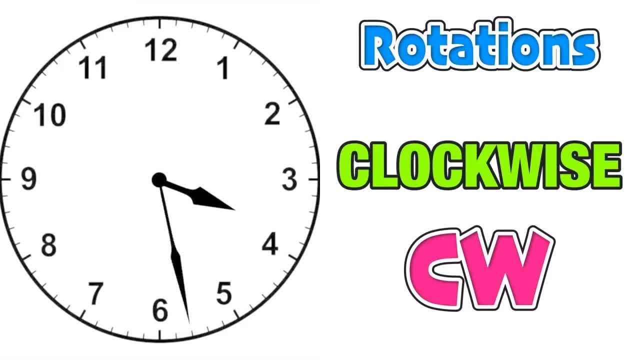 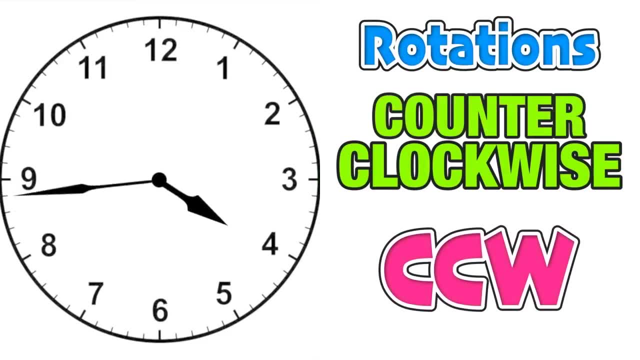 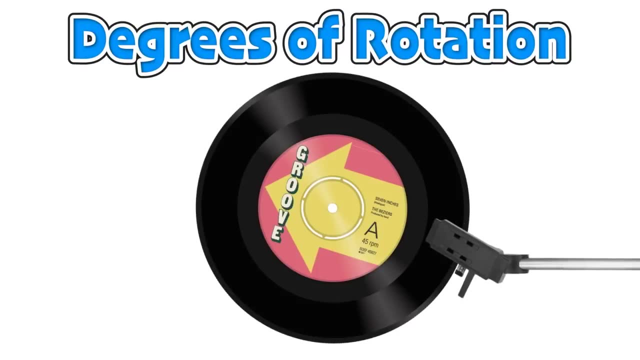 Now we are going to reference two directions for rotations. Clockwise rotations move the same way that the clock does, and counterclockwise rotations just move in the opposite direction that the hand of a clock would normally move. Now, in addition to the direction of a rotation, 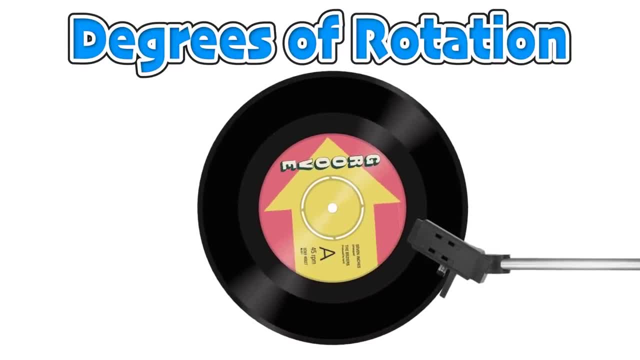 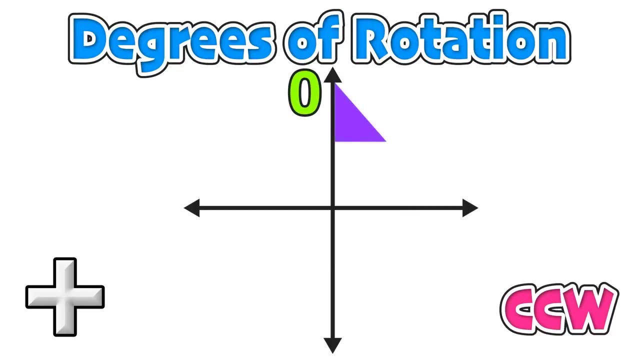 either clockwise or counterclockwise. we are also going to reference rotations in terms of degrees, Just like this circular record. we are moving in a circular rotation, so our degrees are going to be between 0 and 360.. Now, a positive degree of rotation is a counterclockwise movement. So we start with a figure and making 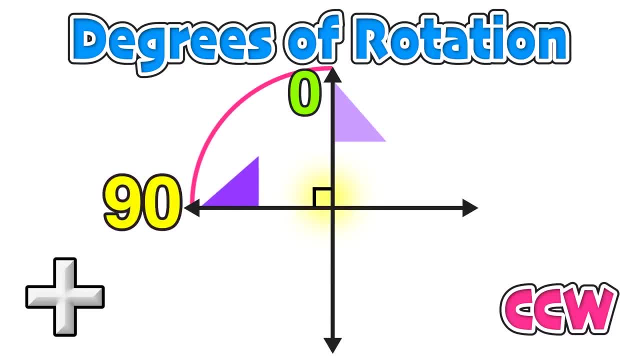 one quarter turn is equivalent to a 90 degree rotation. A second quarter turn is adding another 90 to that, And 90 plus 90 equals 180. So this starts with a 180 degree rotation. A third quarter turn will be adding another 90. This would be a 270 degree rotation. 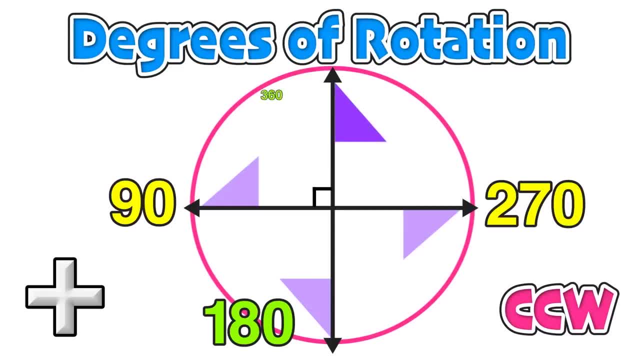 And a final quarter turn brings the figure back to where it started and completes the full 360 degrees. If we rotate in the opposite direction this time, it will end up with a 40 degree rotation, So we are going to start with a 90 degree rotation. 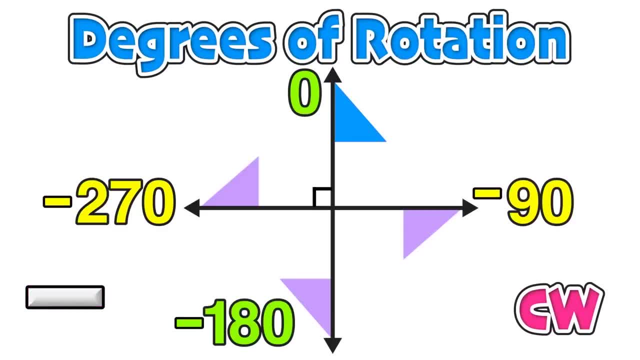 And finally, we are going to reference a rotation. We start by going to the horizontal rotation. In this case we are going to reference a irris rotation which is a 70 degree rotation clockwise. we will see that our rotations will be negative values, so a negative 90. 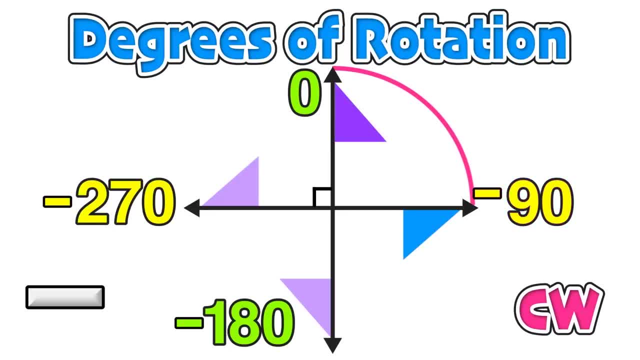 degree rotation is one quarter turn in a clockwise direction. a second quarter turn clockwise would be negative 180, which we notice puts it in the same location as positive 180. so a 180 degree rotation does not matter whether you move clockwise or counterclockwise, you'll end up in the same spot. another. 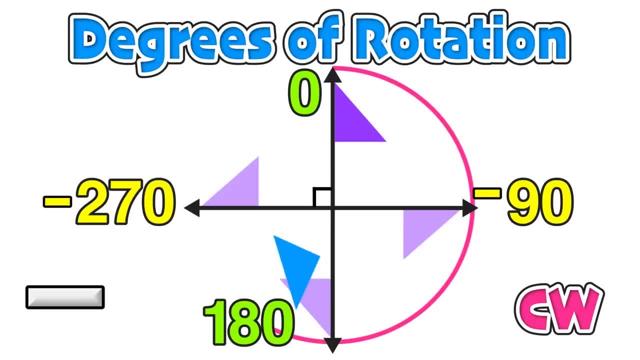 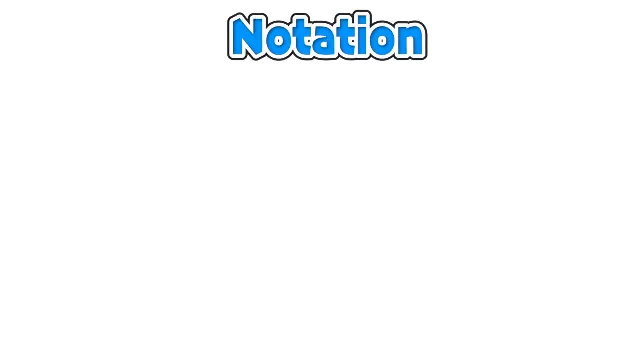 or counterclockwise, you'll end up in the same spot Another quarter turn- clockwise would be negative 270 degrees- and a final quarter turn would complete the 360 degree rotation and bring the figure back to where it started from. Now we will say that rotating a figure is a circular movement around a fixed point. 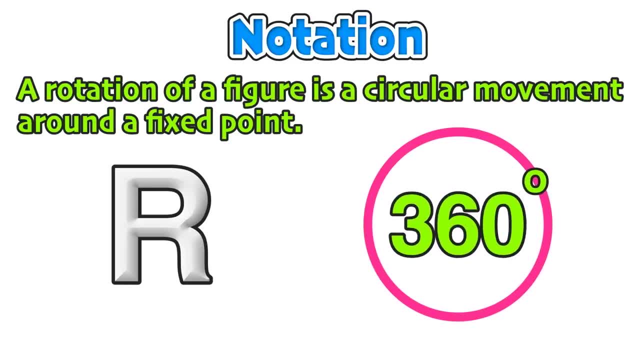 and we use the capital R notation to denote rotations. Remember that when the degrees of notation is a positive number, the rotation is moved in a counterclockwise direction. When the degrees of rotation is a negative number, we move in a clockwise direction. 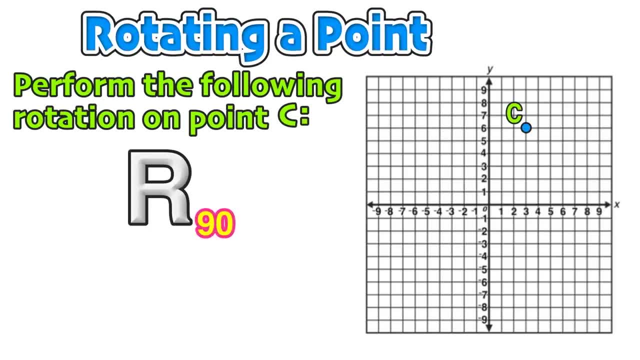 For our first example, we are going to rotate a point. In this case, point C is going to be rotated positive 90 degrees. Since the degrees is a positive number, we will be rotating counterclockwise. We can start by writing down the coordinates of point C at, Since point C lies in the 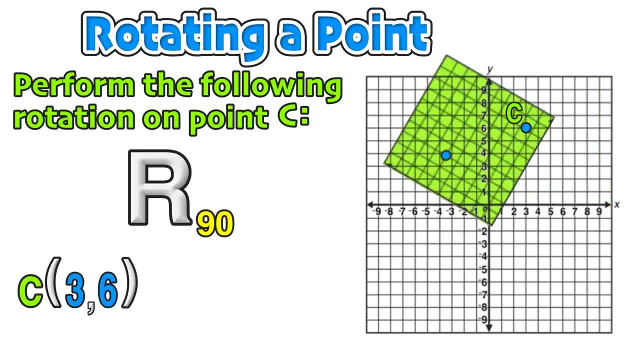 first corner, we can write down the coordinates of point C at. Since point C lies in the first quadrant, we are going to imagine taking that entire quadrant and rotating it one quarter turn. This allows us to find the location of the image C' with coordinates negative. 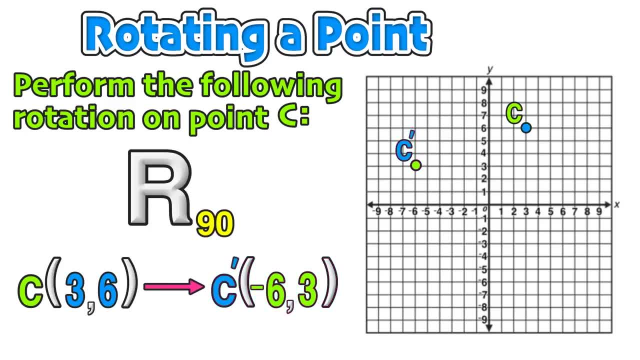 6, positive 3.. Now we can see what if, instead of a 90 degree rotation, it was a positive 180 degree rotation? So in this case we would need two quarter turns of that first quadrant. So the first rotation is the 90 degrees Rotate another quarter turn and we would have a positive 180 degree rotation. 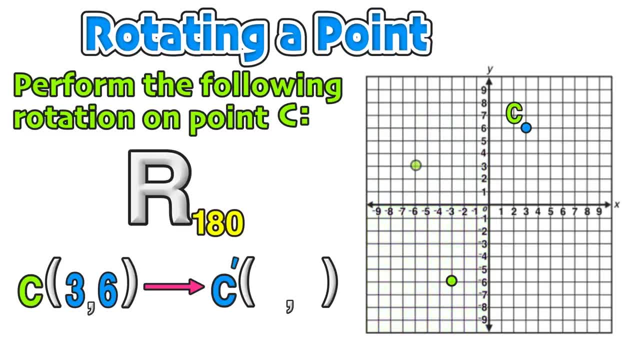 The other quarter turn completes the 180, giving us the coordinates of the new image C' at Now. if the degrees of rotation was 270, we would still complete the same process, but now we would need three quarter turns. So again, start with C in the first quadrant. 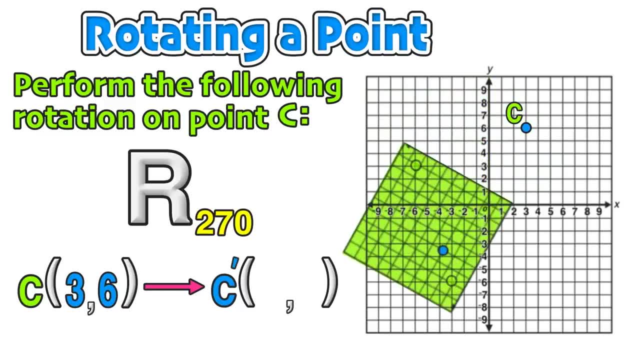 One quarter turn is 90 degrees, A second quarter turn is 180 degrees And a third quarter turn- clockwise- is 270 degrees, giving us the coordinates of the new image C' at positive 6, negative 3.. Now, before we move on, let's just take a moment to visualize what we just did here, when we 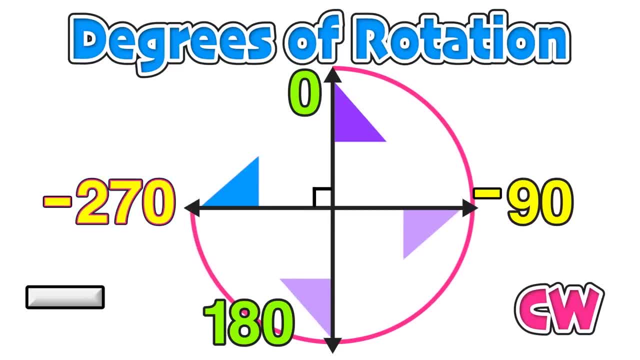 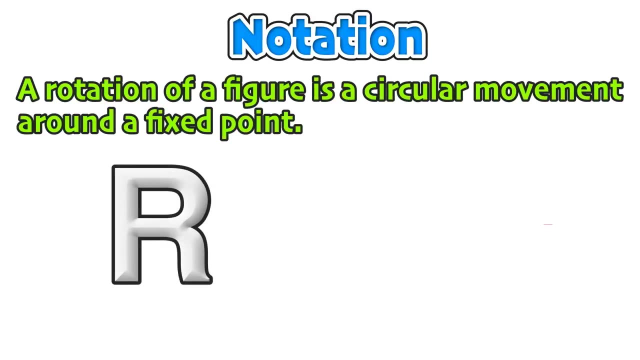 quarter turn clockwise will be negative 270 degrees and a final quarter turn will complete the 360 degree rotation and bring the figure back to where it started. from now we will say that rotating a figure is a circular movement around a fixed point and we use the capital R notation to denote rotations. remember that when 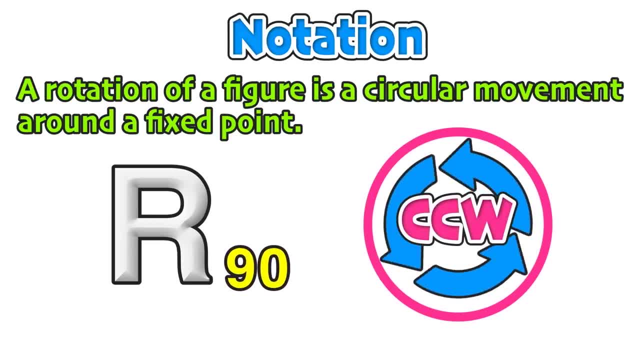 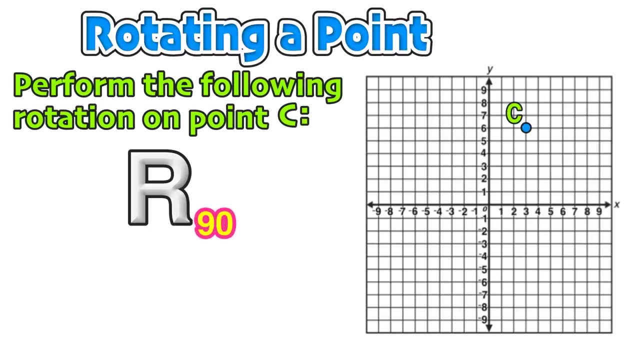 the degrees of notation is a positive number, the rotation is moved in a counterclockwise direction. when the degrees of rotation is a negative number, we move in a clockwise direction. for our first example, we are going to be rotate a point. in this case, point C, is going to be rotated positive 90 degrees, since the 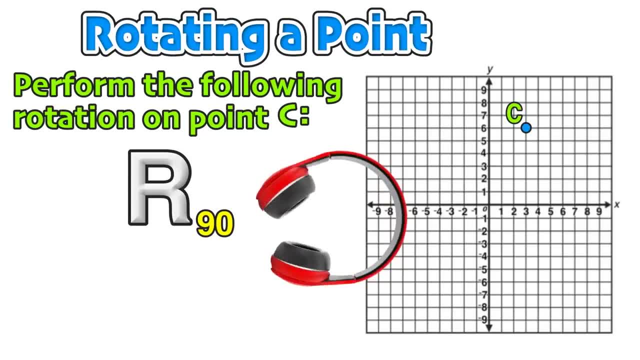 degrees is a positive number. we will be rotating counterclockwise. we can start by writing down the coordinates of point C at 3, 6, since point C lies in the first quarter turn clockwise. we will be rotating counterclockwise. we are going to imagine taking that entire quadrant and rotating it one. 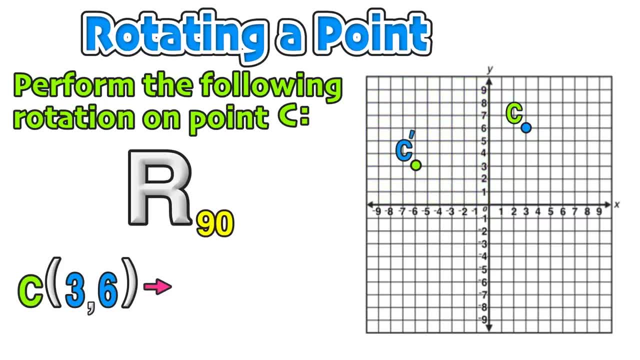 quarter turn. this allows us to find the location of the image C prime with coordinates negative 6, positive, 3. now we can see what if, instead of a 90 degree rotation, it was a positive 180 degree rotation, so in this case, if we would need two quarter turns of that. 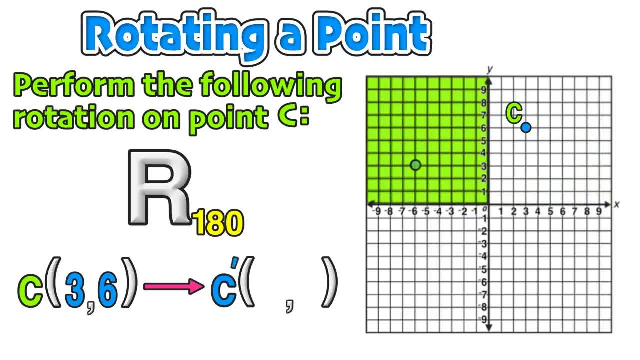 first quadrant. so the first rotation is the 90 degrees. rotate another quarter turn completes the 180, giving us the coordinates of the new image C, prime at negative 3, negative 6. now if the The degrees of rotation was 270, we would still complete the same. 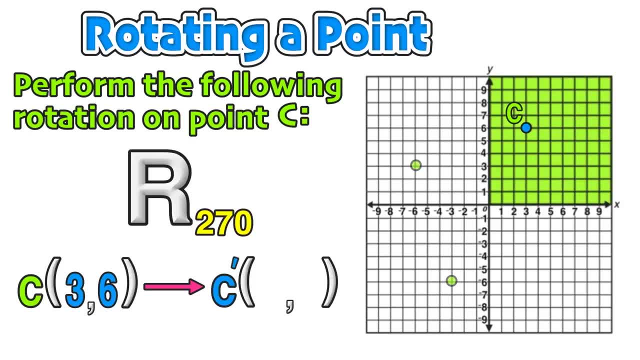 process. but now we would need three quarter turns again. start with C in the first quadrant, if one quarter turn is 90 degrees, a second quarter turn is 180 degrees and a third quarter turn, counterclockwise, is 270 degrees, giving us the coordinates of the new image. C prime at positive 6, negative 3.. 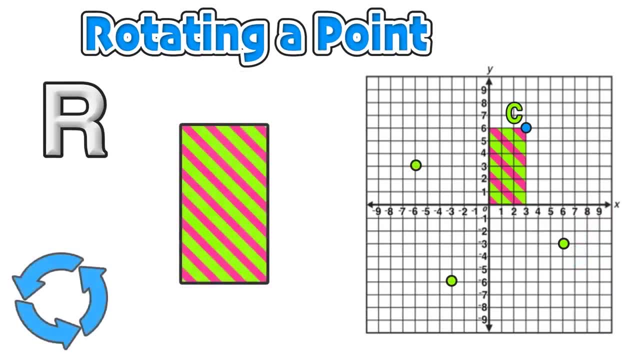 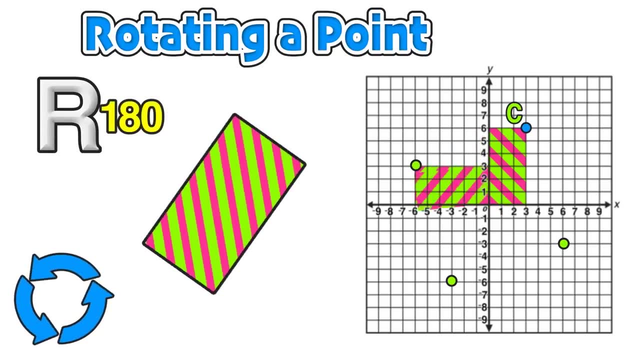 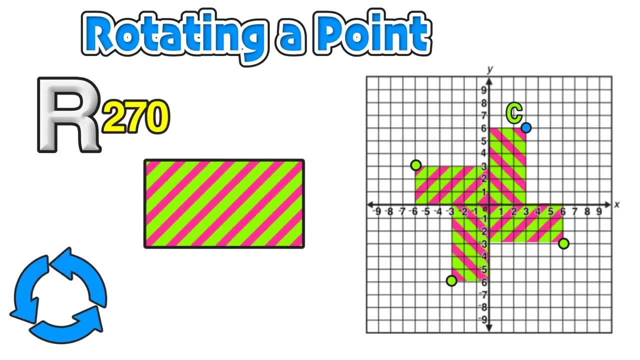 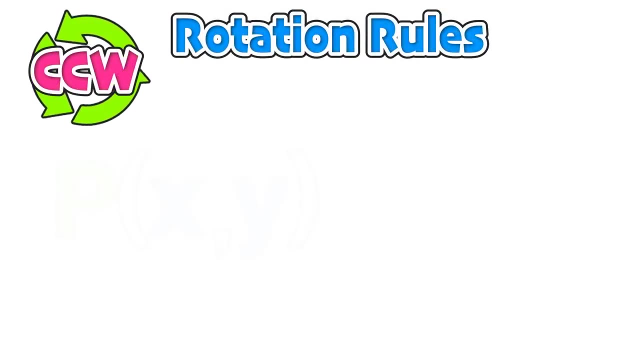 Now, before we move on, let's just take a moment to visualize what we just did here when we rotated this point around the origin. In our last example, we applied a very visual approach to rotating a point around the origin. However, there are some rotation rules that we can also apply. 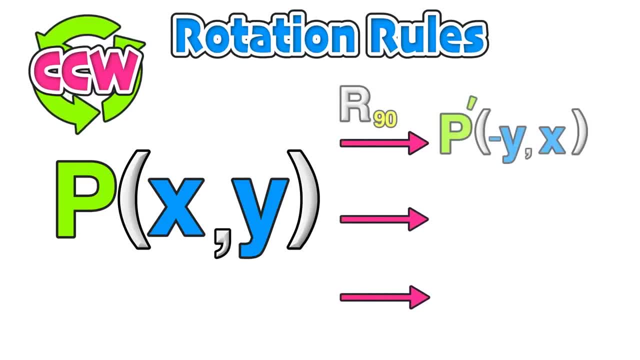 When rotating counterclockwise for any point P with coordinates x, y. there are a set of rules for each type of rotation to find the coordinates of the image. Notice that those negative signs just mean to negate or do the opposite. so positive values will become negative and negative values will become positive. 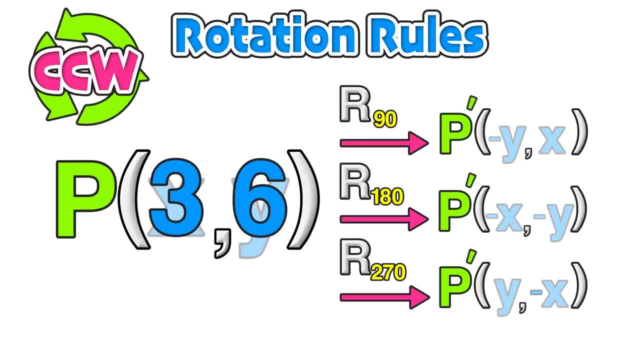 If we apply the point 3, 6 from the last example using these rules, we see that for a 90 degree rotation we would start with the y coordinate negated, so 6 would become negative 6, that's the new x coordinate. 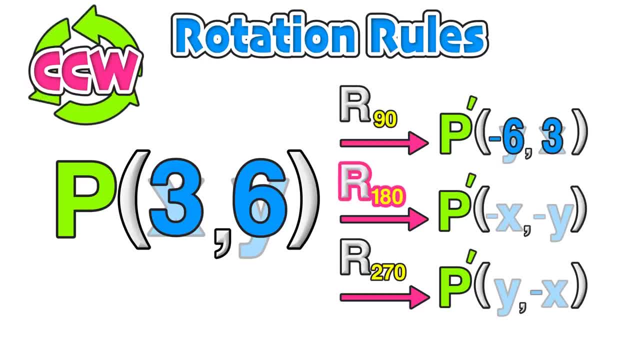 and then the y coordinate is the old x coordinate, which stays the same at positive 3, and we can repeat this process for the rotation of 180 and for the rotation of 270.. Now these points should look very familiar, as they correspond directly to the original x coordinate. 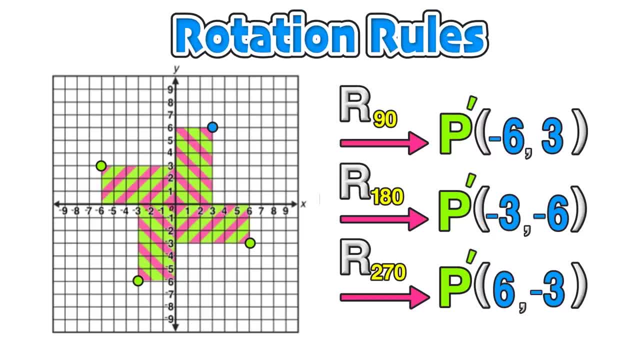 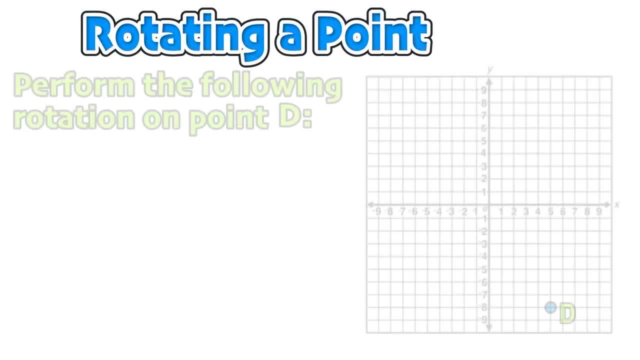 and they are exactly the same as the points we found in the last example, using the visual method. If you don't think that's pretty cool, then I don't know what to say. Okay, moving on to our next example. again, we're going to be rotating a point, in this case a negative degree of rotation. 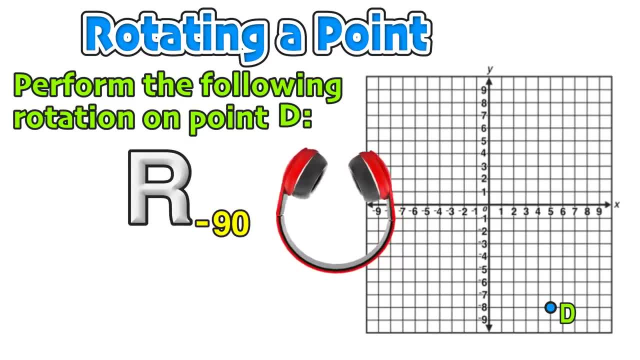 negative 90 degrees means we're moving in a clockwise rotation. We can see that d lies in the fourth quadrant, with coordinates at 5, negative 8. Again, we're going to take a visual approach here. Imagine taking that fourth quadrant with point d contained inside of it. 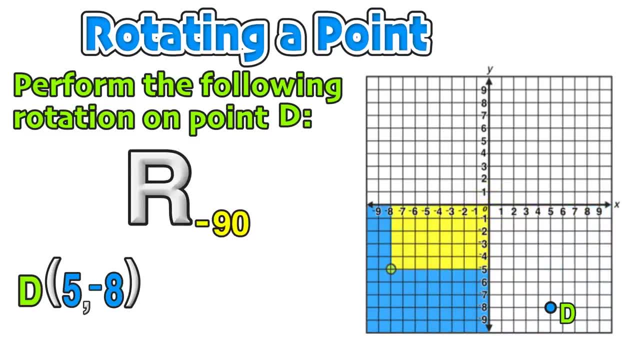 and rotating the entire quadrant, in this case in a clockwise direction. Now we can find the coordinates of the image d prime, with coordinates negative 8, negative 5.. Now let's go ahead and take that same original point d and perform a negative 180 degree rotation. 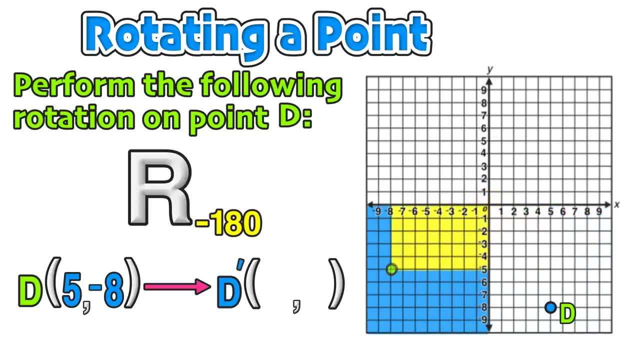 Again, we take that fourth quadrant and we're going to rotate it in a clockwise direction. Now let's go ahead and take that same original point d and perform a negative 180 degree rotation. Again we take that fourth quadrant. one quarter turn clockwise is negative 90,. 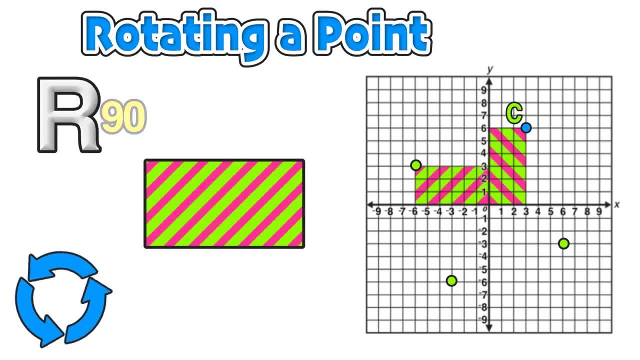 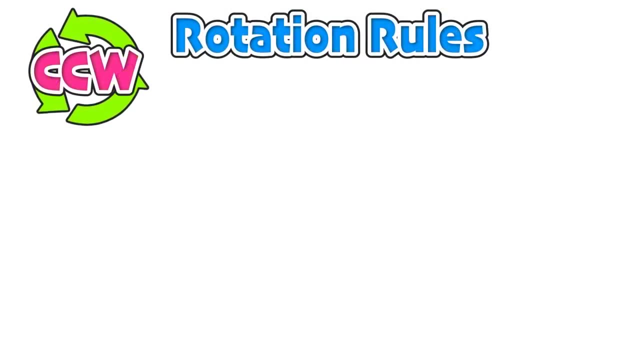 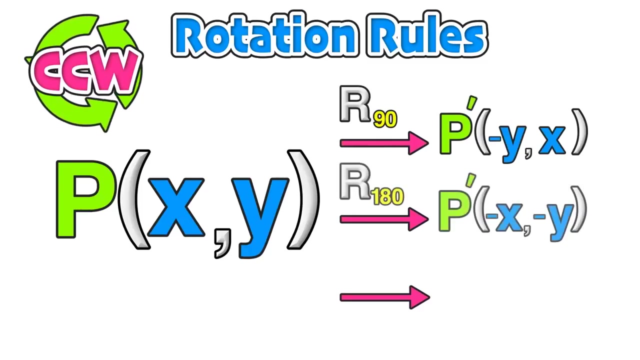 rotated this point around the origin. In our last example, we applied a very visual approach to rotating a point around the origin. However, there are some rotation rules that we can also apply When rotating counterclockwise for any point P with coordinates. there are a set of rules for each type of rotation. 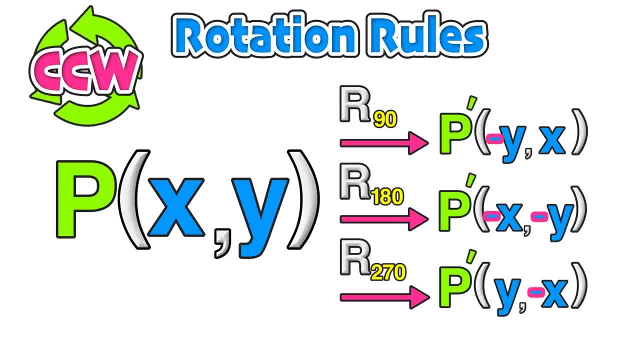 to find the coordinates of the image. Notice that those negative signs just mean to negate or do the opposite. So positive values would become negative and negative values would become positive. If we apply the point from the last example using these rules, we see that for a 90 degree. 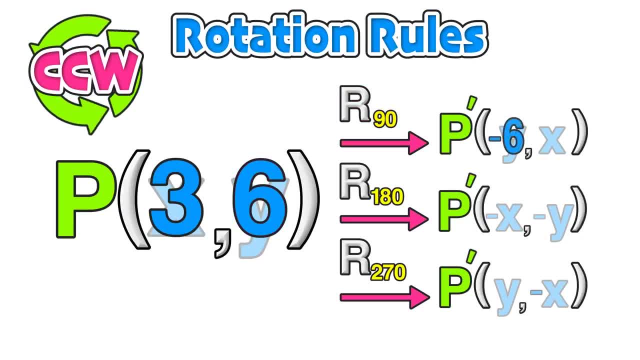 rotation, we would start with the y coordinate negated, so 6 would become negative 6, that's the new x coordinate, And then the y coordinate is the old x coordinate, which stays the same at positive 3.. And we can repeat this process for the rotation of 180 and for the rotation 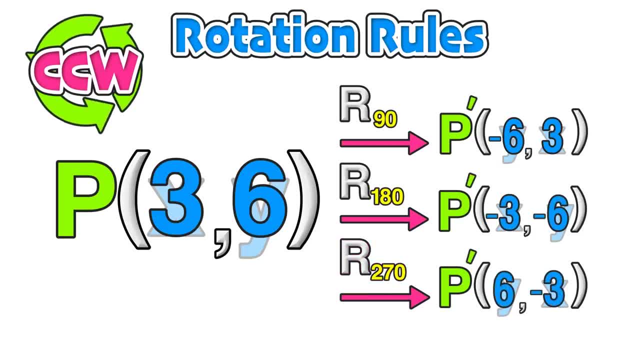 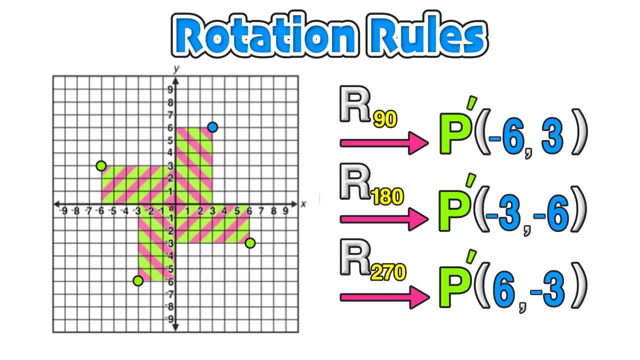 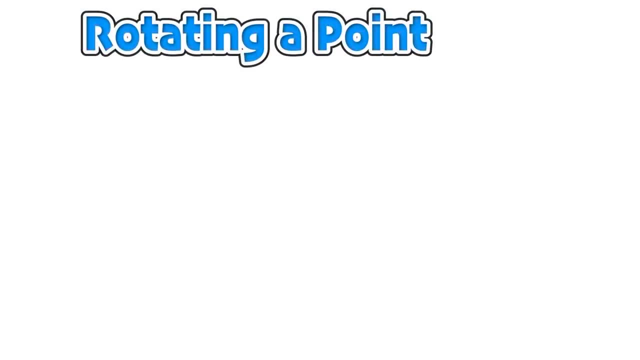 of 270.. Now these points should look very familiar, as they correspond directly with the points that we found in the last example, using the visual method. If you don't think that's pretty cool, then I don't know what to say. Okay, moving on to our next example. Again, we're going to be rotating a point in this. 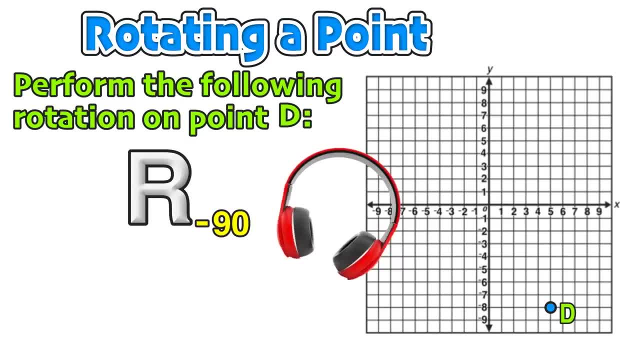 case a negative degree of rotation. Negative 90 degrees means we're moving in a clockwise rotation. We can see that d lies in the fourth quadrant, with coordinates at 5, negative 8.. Again, we're going to take a visual approach here. 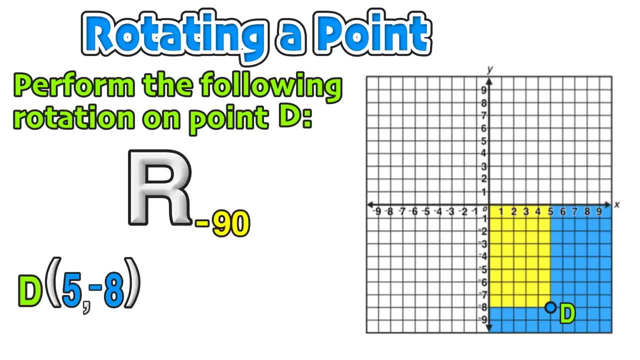 Imagine taking that fourth quadrant with point d contained inside of it and rotating the entire quadrant, in this case in a clockwise direction. Now we can find the coordinates of the image d prime, with coordinates negative 8,, negative 5.. Now let's go ahead and take that same original point d and perform a negative 180 degree rotation. 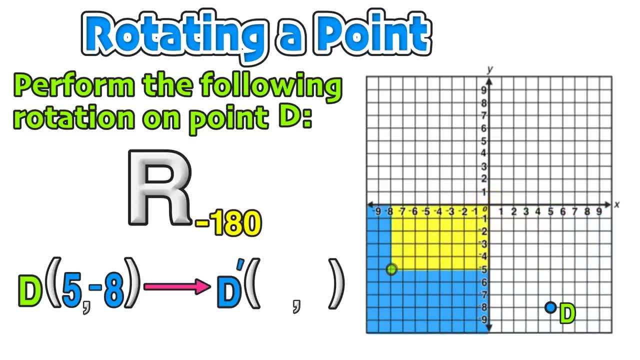 Again we take that fourth quadrant. one quarter turn clockwise is negative 90, a second quarter turn would be negative 180.. Now again we can find the coordinates of the image d prime at negative 5, positive 8.. Now we'll take a look at what would happen if, instead of a negative 180 rotation, it was a negative 270.. 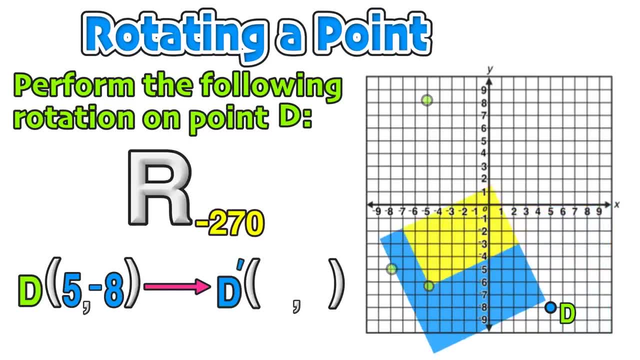 Again. so we're going to take a visual approach here. We can start with d. in that fourth quadrant one quarter turn is the negative 90, a second quarter turn is negative 180.. We need one more third quarter turn to get to negative 270 with the image d prime at positive 8, positive 5.. 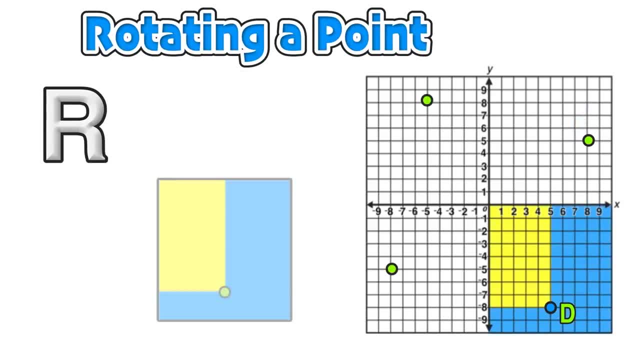 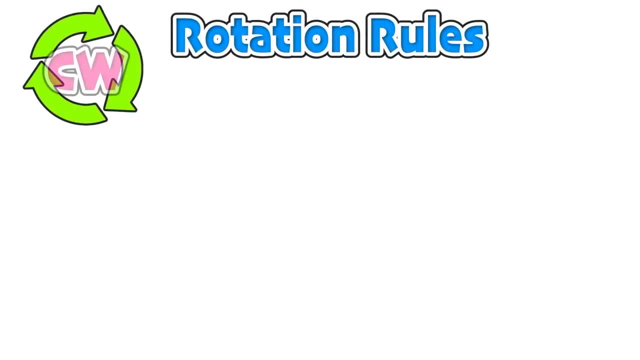 Now that we have completed all of the degrees of rotation in a clockwise direction, let's go ahead and visualize what we did on that last example. Now, just as we had rotation rules for counterclockwise rotations, we have another set of rules for clockwise rotations. 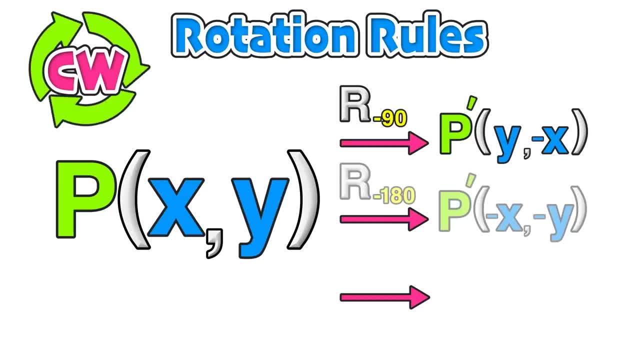 So for any point P with coordinates x, y, we have a set of rules for negative 90,, negative 180, and negative 270.. And again, those negative signs just mean to negate or to switch the sign. So if we use the point from the last example, 5,, negative 8.. 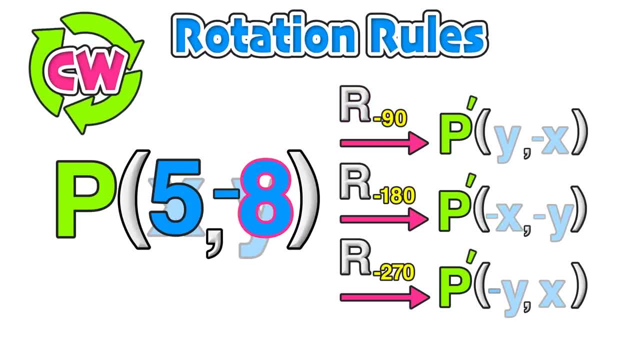 By applying the negative sign to negative 180,, negative 270.. By applying the negative 90 degree rule, we start with the y coordinate, negative 8.. And then the second value is the negated x coordinate, so negative 5.. 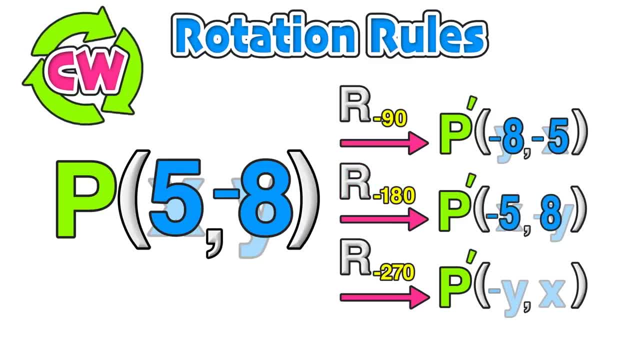 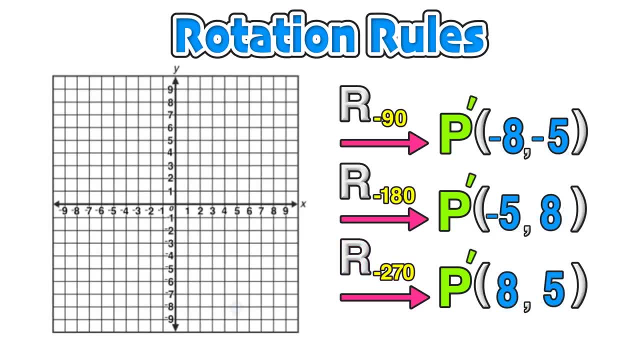 Now you can go ahead and apply these rules for negative 180 as well as for negative 270 to get the coordinates of those images. Now again, these points should look familiar because they correspond with the points that we found in the last example using the visual method. 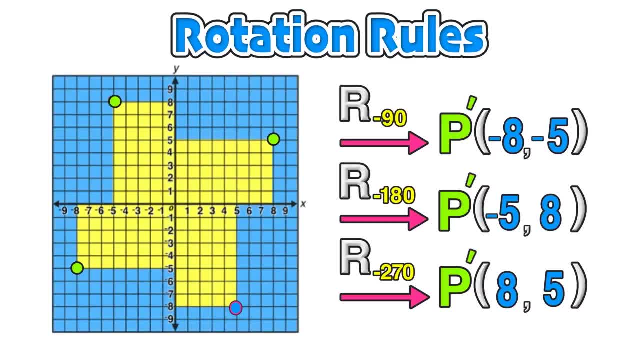 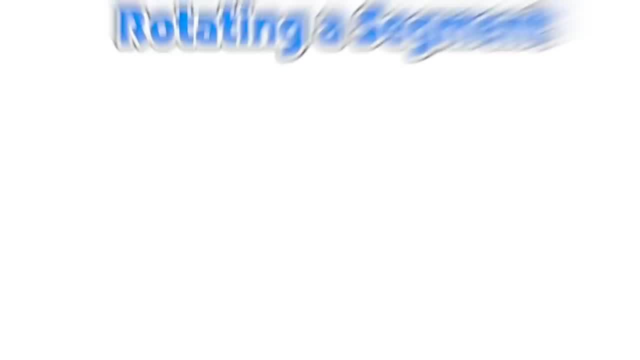 So, basically, it's up to you to decide Which method you want to use. They each work effectively, But if you're going to use the rules, you're going to have to memorize them, Okay, so now we're going to step it up and take a crack at rotating a line segment. 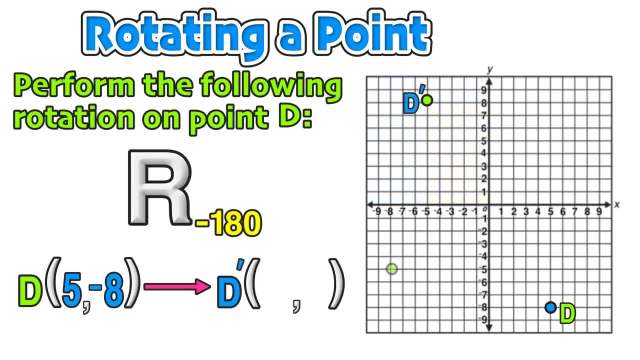 a second quarter turn would be negative 180.. Now again, we can find the coordinates of the image d prime at negative 5, positive 8.. Now we'll take a look at what would happen if, instead of a negative 180 rotation, it was: 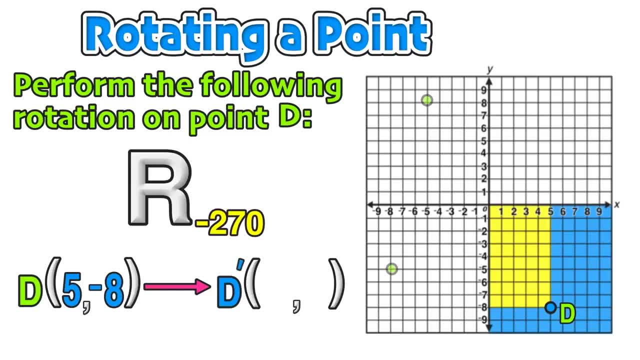 a negative 270.. Again, start with d in that fourth quadrant. one quarter turn is the negative 90,. a second quarter turn is negative 180.. We need one more third quarter turn To get to negative 270, with the image d prime at positive 8, positive 5.. 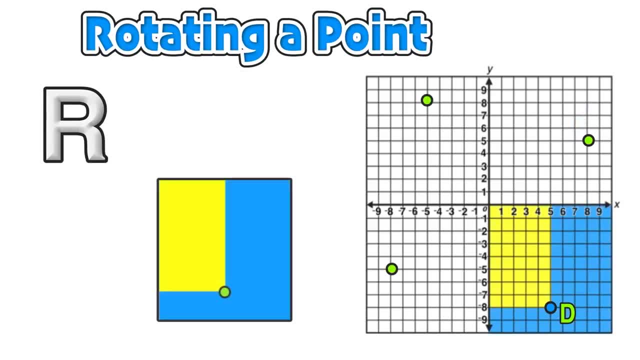 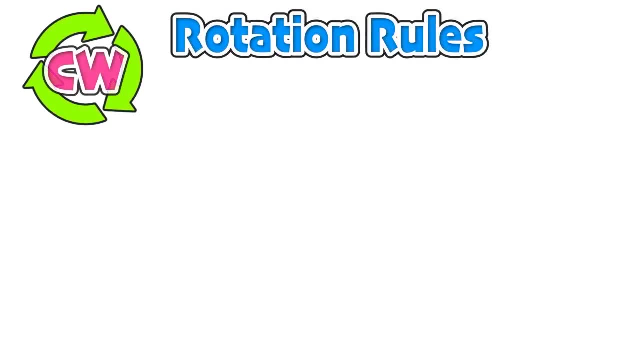 Now that we have completed all of the degrees of rotation in a clockwise direction, let's go ahead and visualize what we did on that last example. Now, just as we had rotation rules for counterclockwise rotations, we have another set of rules for. 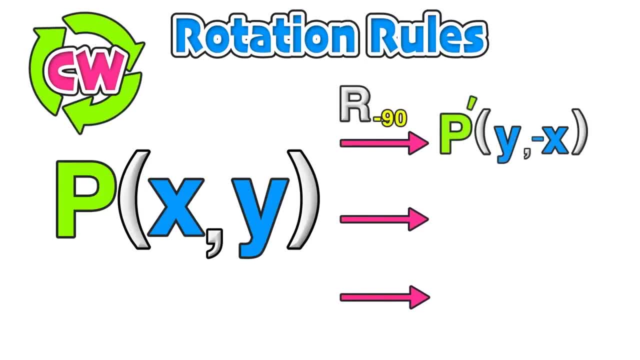 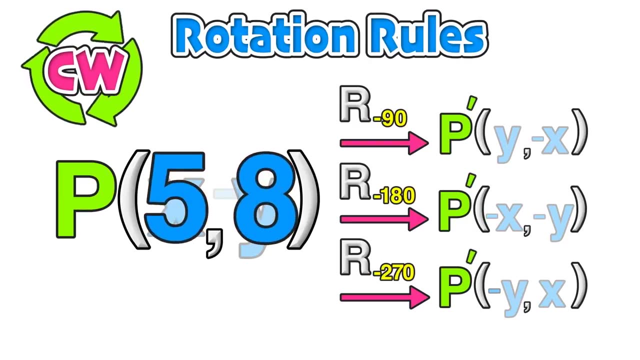 clockwise rotations. So for any point p with coordinates x, y, we have a set of rules for negative 90,, negative 180, and negative 270.. And again, those negative signs just mean to negate or to switch the sign. So if we use the point from the last example- 5,, negative 8, by applying the negative 90, 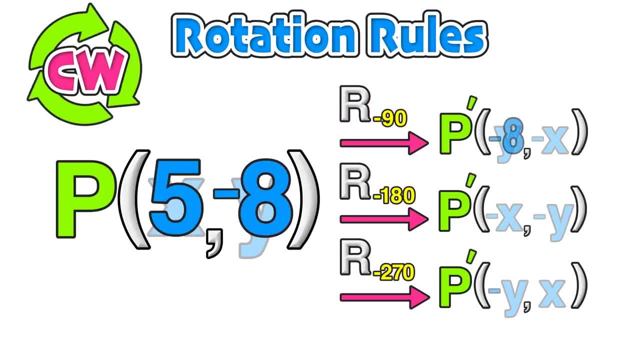 degree rule. we start with the y coordinate- negative 8,- and then the second value is the negated x coordinate, so negative 5. Now you can go ahead and apply these rules for negative 180 as well as for negative 270. 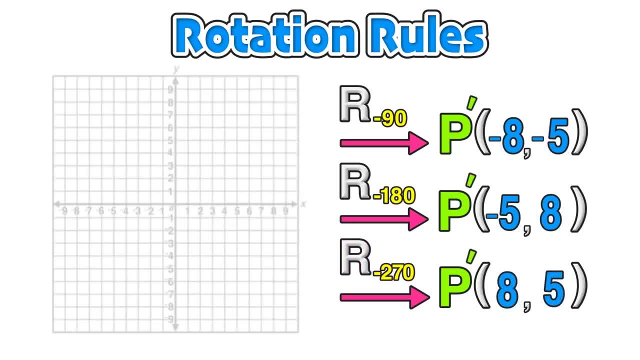 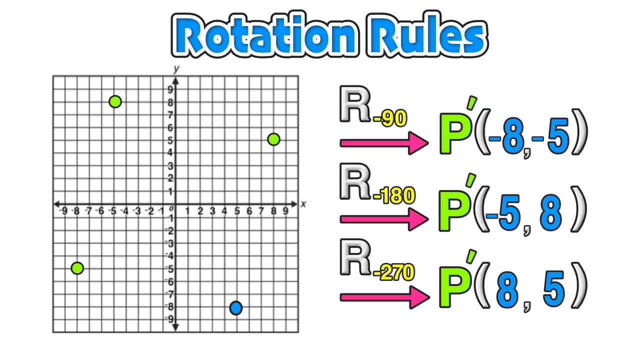 to get the coordinates of those images. Now again, these points should look familiar because they correspond with the points that we found in the last example using the visual method. So, basically, it's up to you to decide which method you want to use. they each work effectively. 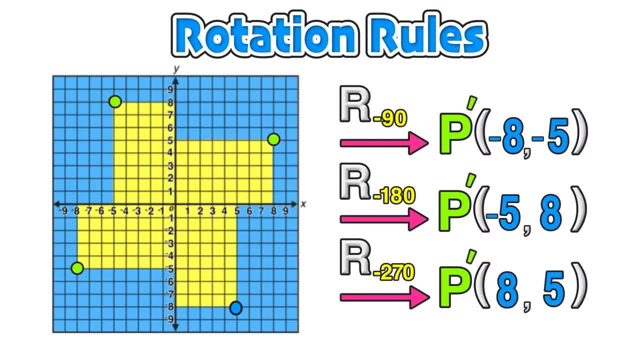 but if you're going to use the rules, you're going to have to memorize them. Okay, So now we're going to step it up. Okay, So we're going to step it up and take a crack at rotating a line segment. 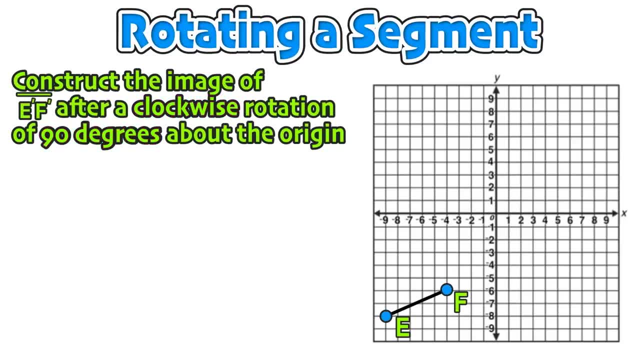 In this case we want to construct E prime, F prime after a clockwise rotation of 90 degrees, so that would be a negative 90 degree rotation. Now we can start by writing down the coordinates of the endpoints E and F and we want to find: 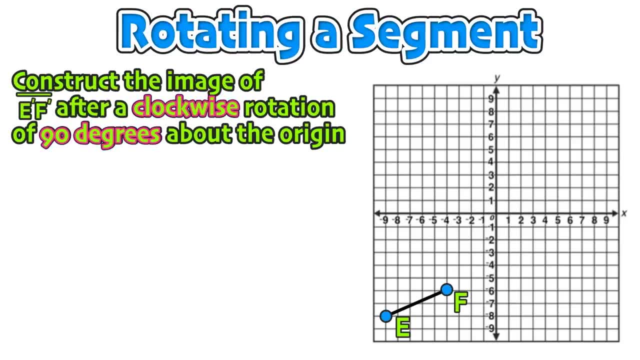 In this case we want to construct E prime, F prime after a clockwise rotation of 90 degrees. So that would be a negative 90 degree rotation. Now we can start by writing down the coordinates of the endpoints E and F, And we want to find the coordinates of the endpoints E and F. 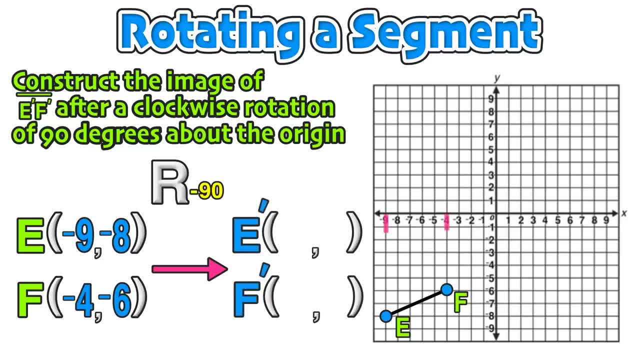 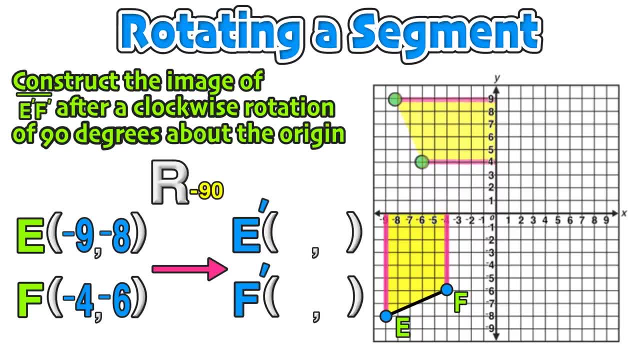 this allows us to find the location of the new line segment e prime, f prime. once we construct the segment, we can see that e prime is at negative eight nine and that f prime is at negative six four. so basically, all that we did was take that line, segment ef, and rotate it one quarter turn. 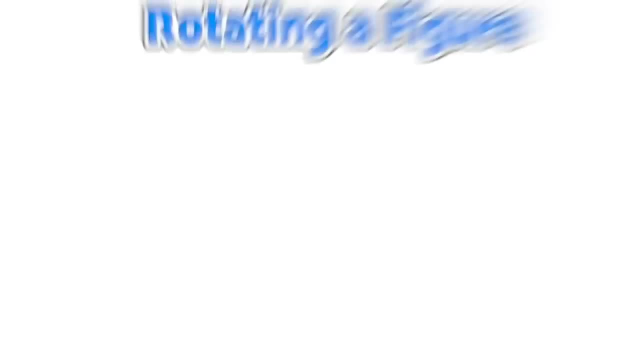 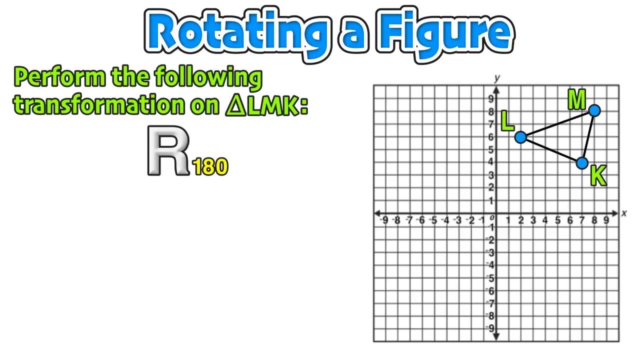 clockwise about the origin and for our final example, we're going to take a shot at rotating a figure, in this case a positive 180 degrees. so we start by writing down the coordinates of the vertices of triangle l, m, k, and we're looking to find the coordinates of the image of point l. 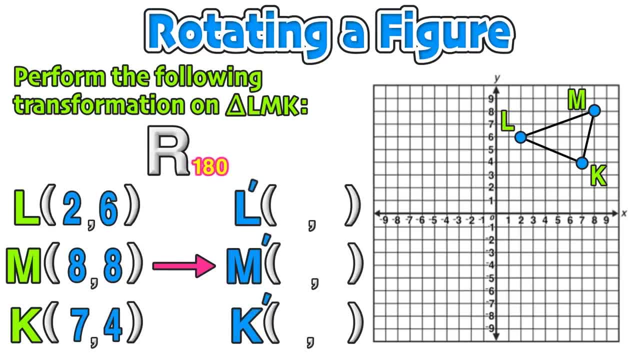 prime, m prime and k prime. now, since it's a positive 180 degrees, we're going to take this figure and rotate it two quarter turns in a counterclockwise direction to get it to its final location. however, if we actually made a mistake here and went the wrong way, going clockwise, 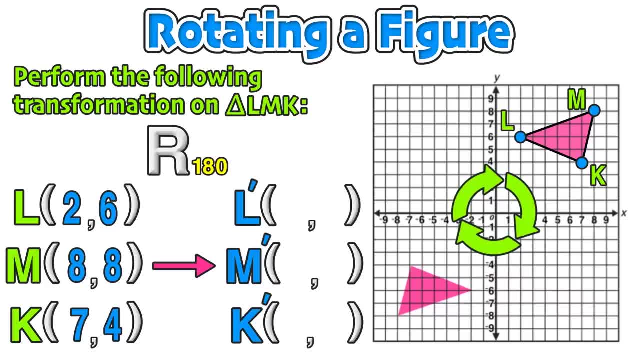 we're going to have to rotate it one quarter turn in a counterclockwise direction to get it to its final location. we see that we would end up in the same spot. so if you remember from earlier, for 180, it doesn't matter whether you go clockwise or counterclockwise, you'll still end up in the same. 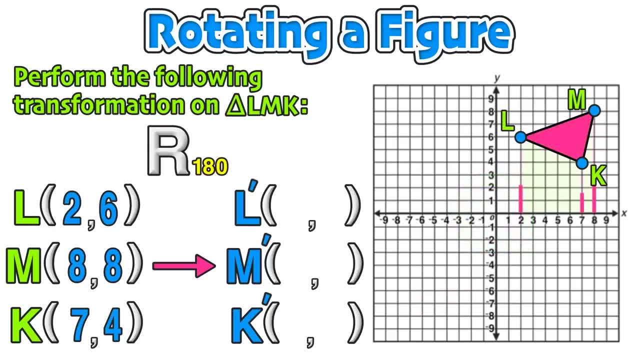 position. now, using our visual approach, we construct three reference lines and we're going to go ahead and rotate that entire quadrant. two quarter turns in a counterclockwise direction. now we can construct the image of the new figure, identify l prime, k prime and m prime, l prime with coordinates at negative 2, negative 6. 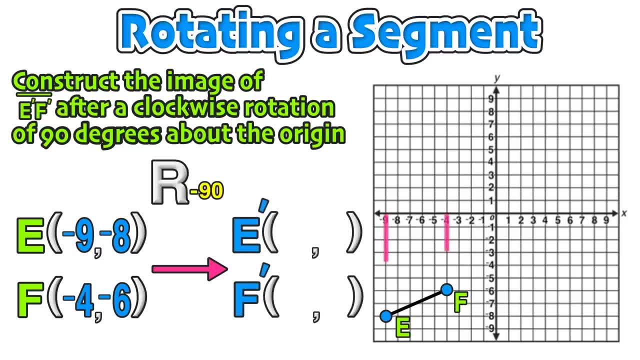 the coordinates of the image of E prime and F prime. So again, we just want to take the entire quadrant that EF is in and rotate it one quarter turn clockwise. This allows us to find the location of the new line. segment E prime, F prime. 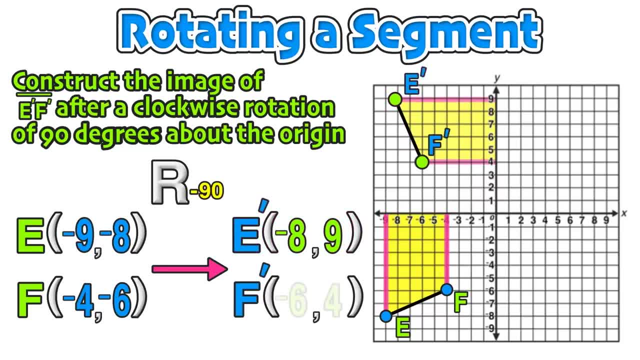 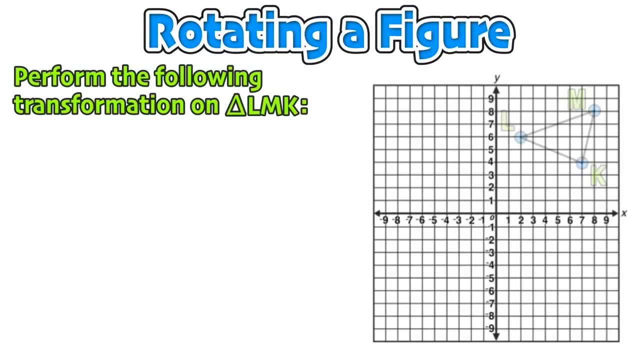 Once we construct the segment, we can see that E prime is at negative eight nine and that F prime is at negative six four. So basically all that we did was take that line, segment EF, and rotate it one quarter turn clockwise about the origin. 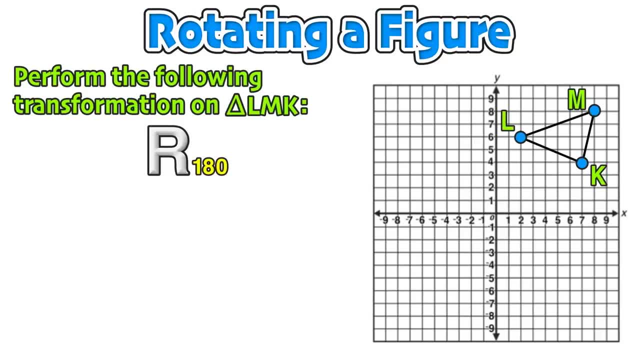 And for our final example, we're going to take a shot at rotating a figure, in this case a positive 180 degrees. Okay, We start by writing down the coordinates of the vertices of triangle LMK and we're looking to find the coordinates of the image of point L prime, M prime and K prime. 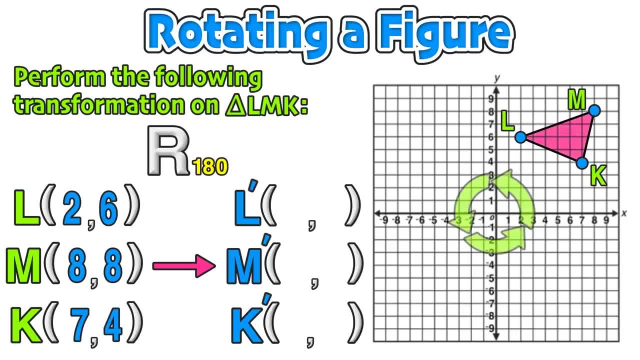 Now, since it's a positive 180 degrees, we're going to take this figure and rotate it two quarter turns in a counterclockwise direction to get it to its final location. However, if we actually made a mistake here and went the wrong way- going clockwise, we 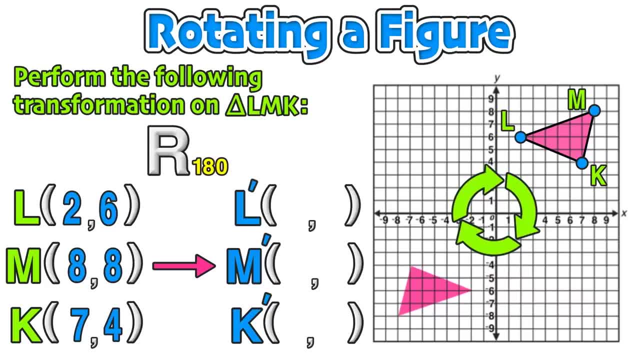 see that we would end up in the same spot. So, if you remember from earlier, for 180, it doesn't matter Whether you go clockwise or counterclockwise, you'll still end up in the same position. Now, using our visual approach, we construct three reference lines and we're going to go. 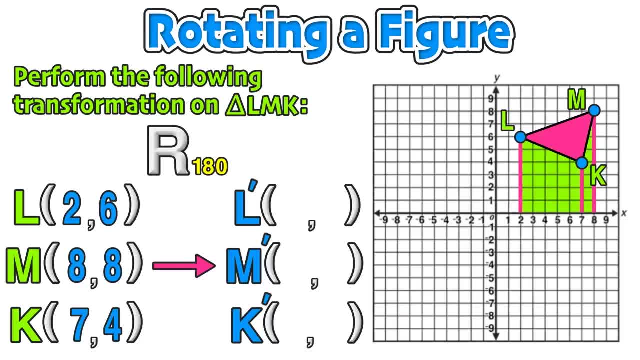 ahead and rotate that entire quadrant. two quarter turns in a counterclockwise direction. Now we can construct the image of the new figure, identify L prime, K prime and M prime. L prime with coordinates at negative eight. M prime with coordinates at negative. two negative six. 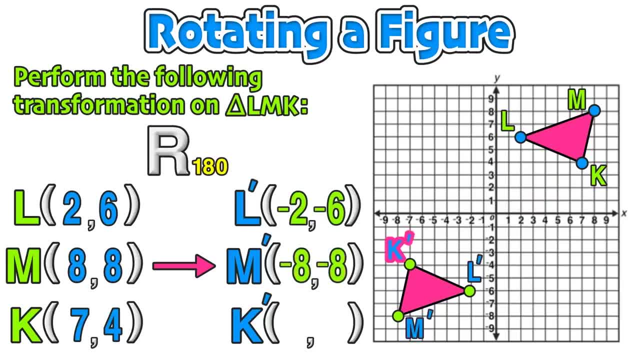 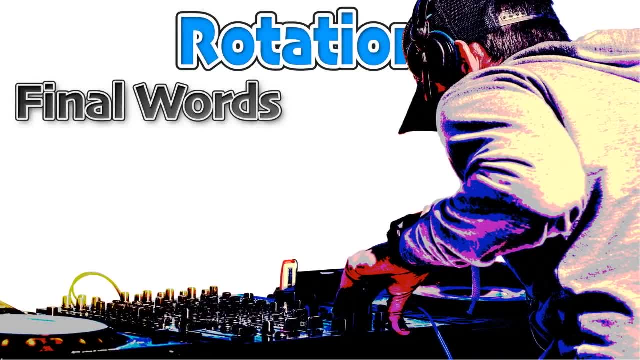 M prime at negative eight negative eight And K prime at negative seven negative four. And now for our final words on rotations. A rotation is a circular turn around a fixed point. We also say that a rotation is a change in a figure's orientation.